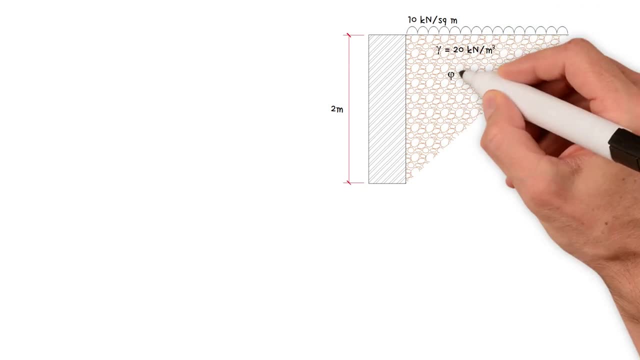 20 kilonewtons per cubic meter and an angle of friction of 30 degree. The water table is 4.5 meters below the top of the retained surface. So how can we calculate the characteristic loads and their location generated by the 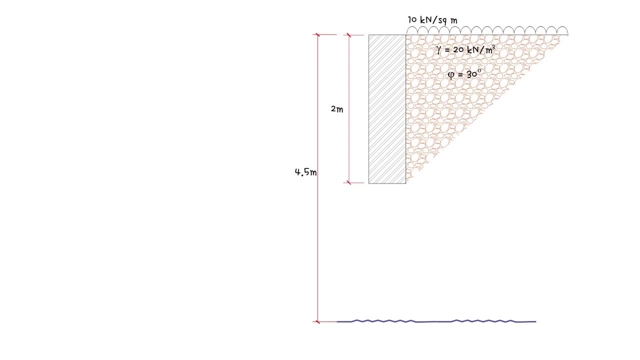 retained soil behind the wall. Also, how can we calculate the ultimate loads for designing the wall? First of all, we need to work out the coefficient of active pressure, which equals 1 minus sine soil friction angle 30, divided by 1 plus sine soil friction angle 30. This gives 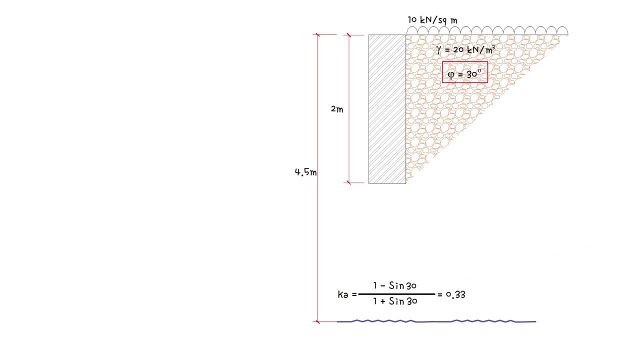 us a value of 0.3.. Next, working out the active pressure at the base of the wall, which equals the coefficient of active pressure, 0.33, times the soil density, 20 kilonewton per cubic meter times the height. 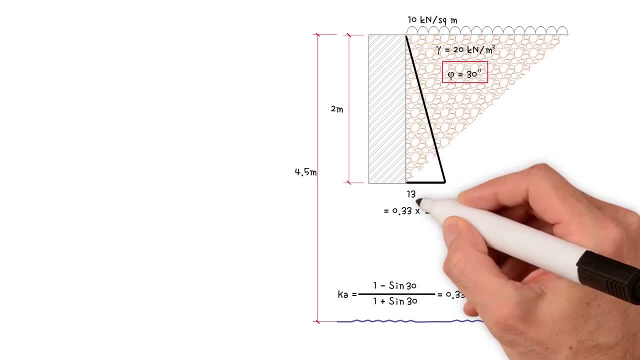 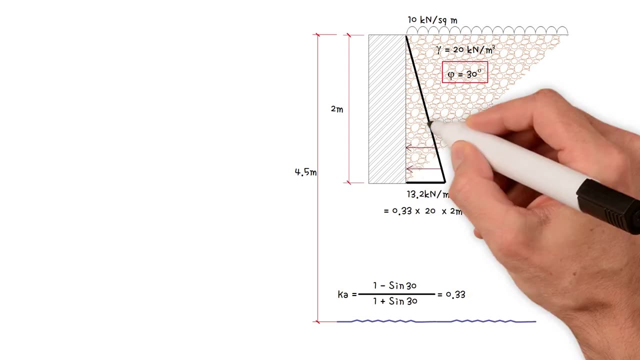 2 meters. This gives us a value of 13.2 kilonewtons per meter per meter run. Therefore, for a triangular distributed load, the magnitude of the resultant force P is the area of the triangle, which is 0.5, times 13.2 kilonewtons per meter per meter, times the depth: 2 meters. 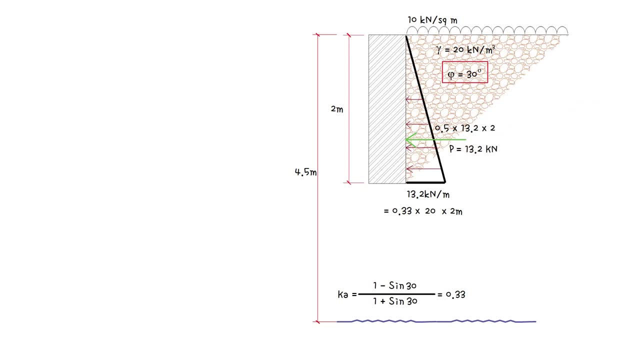 This gives us a value of 13.2 kilonewtons per meter run. The force of triangle acts about one third of the length of triangle, So this is the location of the resultant force P For a rectangular distributed load. the magnitude of the resultant force Q is a coefficient. force Q is equivalent to the area of the rectangle, which is 10 kilonewtons per square meter surcharge times the depth: 2 meters. This gives us a value of 20 kilonewtons per meter run. The force of rectangle acts in the middle of the length of rectangle. 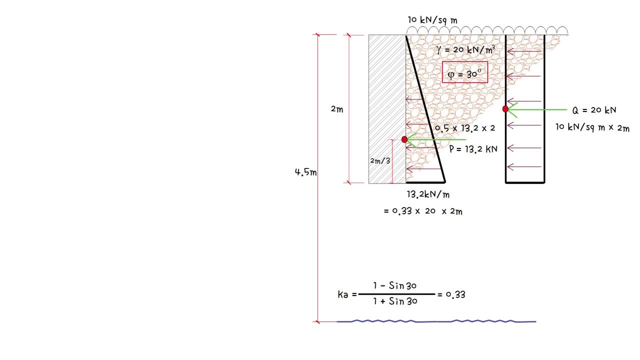 So this is the location of the resultant force Q. Next, we need to work out the ultimate load combinations for designing the wall. Bear in mind that partial factors for loads originating from pressures due to retained materials vary depending on the type of analysis being carried out. 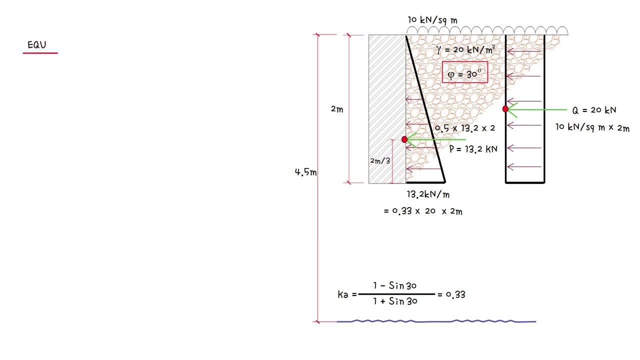 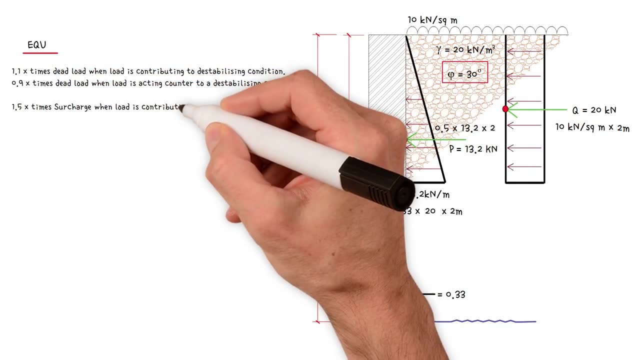 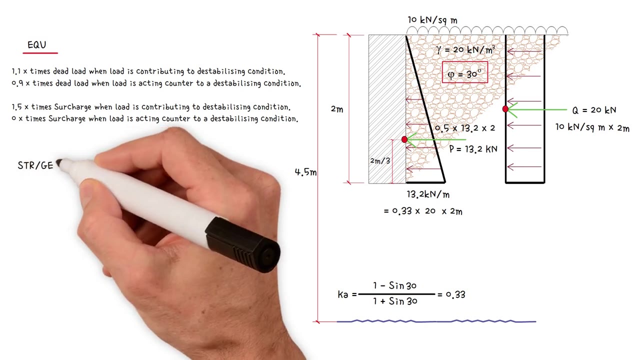 In the case of checking for equilibrium, the following partial factors apply to dead and imposed loads When designing the retaining structure. EN 1990, offers three approaches with respect to the application of partial factors. The UK National Annex to EN 1990, states that approach 1 is adopted. 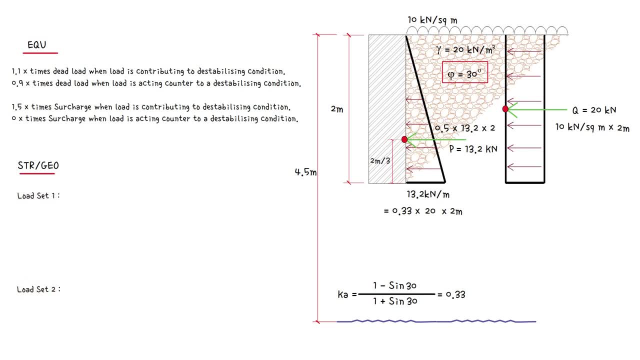 In this approach, two load combinations known as sets are considered. Load set: 1. 1.35 times dead load when load is contributing to destabilizing condition. One times dead load when load is acting against the plane. 1.35 times dead load when load is contributing to destabilizing conditions. One times dead load when load is acting against the plane. One times dead load when load is acting against the plane. One times dead load when load is acting against the plane. 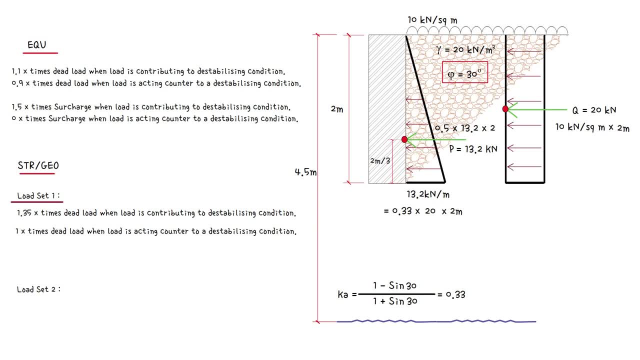 consumption jawthree sense pyramid 20173.. A 2016,. early industrial structure revealed the response: 2 times continuous killed capacity. w1, macroning of the announced' light andום girth socialah c4service. counter to a destabilizing condition: 1.5 times surcharge when load is. 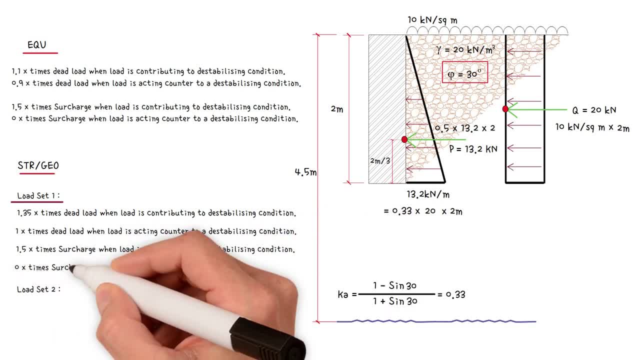 contributing to destabilizing condition: 0 times surcharge when load is acting counter to a destabilizing condition. for load set to 1 times dead load when load is contributing to destabilizing condition: 1.3 times surcharge when load is contributing to destabilizing condition. 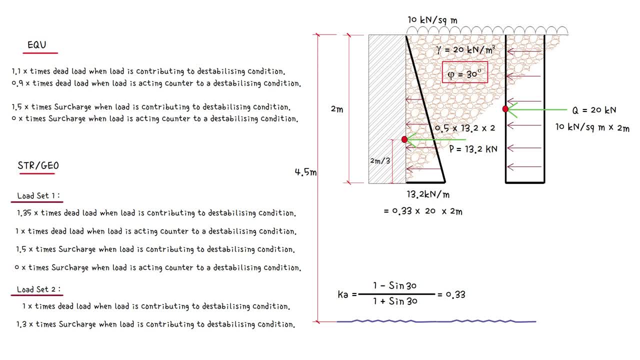 so back to our worked example to calculate the ultimate loads for designing the wall. we would have load set 1, 1.35 times 13.2, which equals 17.8, 2 kilonewtons per metre, and 1.5 times 20, which equals 30 kilonewtons per metre. 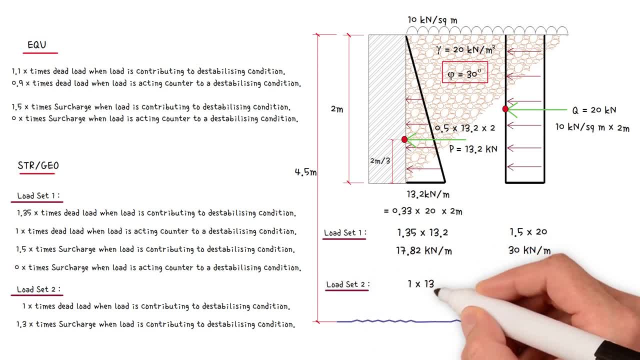 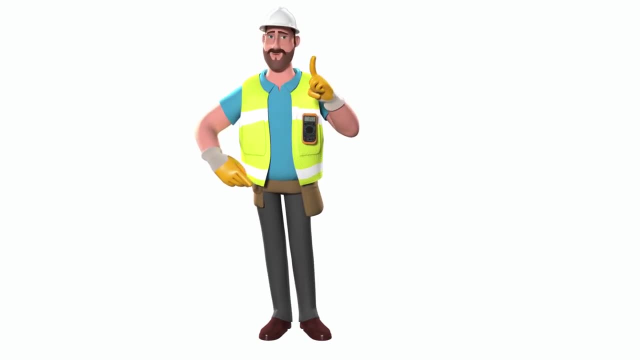 for load set: 2: 1 × 13.2 equals 13.2 kilonewtons per meter, and 1.3 × 20,, which equals 26.. Thanks for watching. We hope you found some useful tips. Check out our website at structuralengineercalcscom.